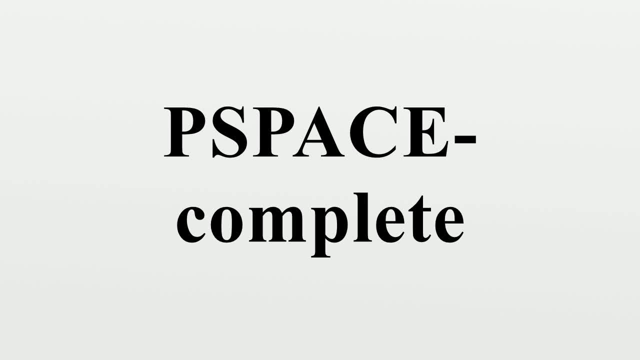 When N is the input size and K is the number of states. GP. the first known PSPACE complete problem was the word problem for deterministic context-sensitive grammars. In the word problem for context-sensitive grammars one is given a set of grammatical transformations which can increase. 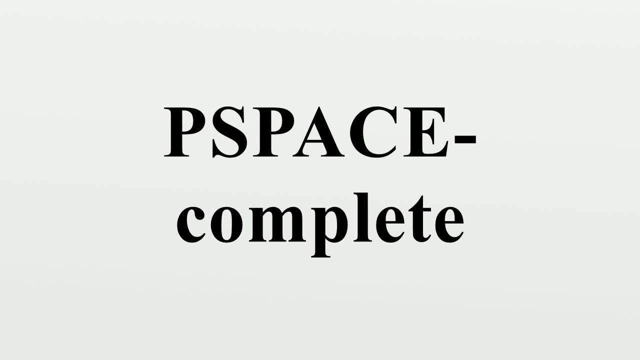 the length of a sentence and wishes to determine if a given sentence could be produced by these transformations. 坌 With our experience진 c speaking. P allocation system, department metal. The technical condition of determinism ensures that this process can be solved in polynomial space. 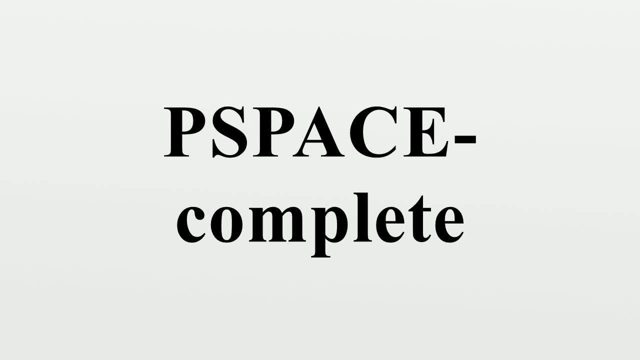 Encourada showed that every program computable in linear space could be converted into the parsing of a context-sensitive grammar in a way which preserves determinism. In 1970, Savage's theorem showed that PSPACE is closed under non-determinism. 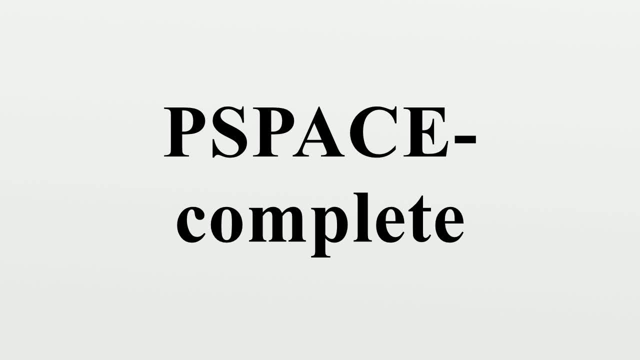 implying that even non-deterministic, context-sensitive grammars are, in PSPACE, Quantified Boolean Formulas. Nowadays, The archetypal PSPACE complete problem is generally taken to be the quantified Boolean formula problem, a generalization of the first known NP-complete problem, the Boolean satisfiability problem. 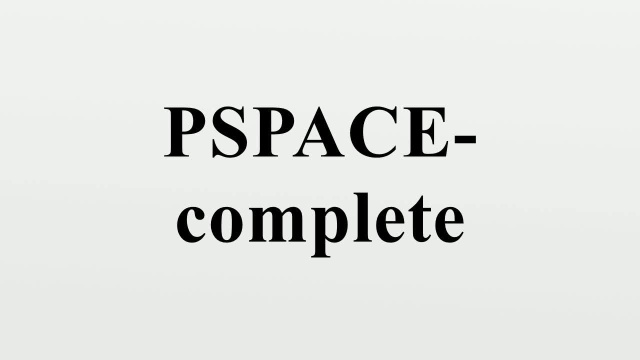 The satisfiability problem is the problem of whether there are assignments of truth values to various Boolean formulas. There are variables that make a Boolean expression true, For example. one instance of SAT would be the question of whether the following is true: The quantified Boolean formula problem differs in allowing both universal and existential quantification over the values of the variables. 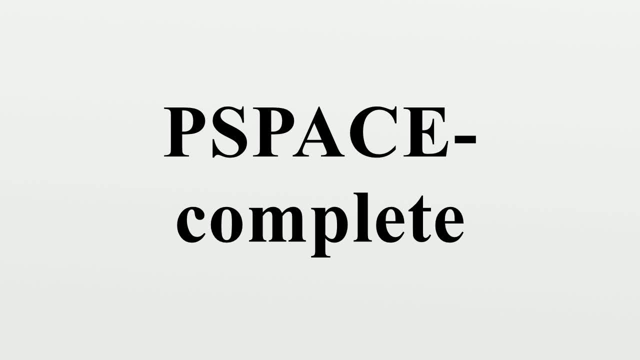 The proof that QBF is a PSPACE complete problem is essentially a restatement of the proof of Savage's theorem in the language of logic and is a bit more technical. Puzzles and Games. The NP-complete problem in the previous section resembles typical puzzles. 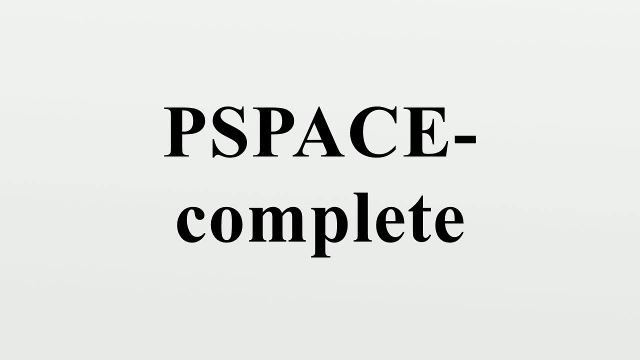 Is there some way to plug in values? that solves the problem Correspondingly. the PSPACE complete problem there resembles games. Is there some move I can make such that for all moves my opponent might make, there will then be some move I can make to win?